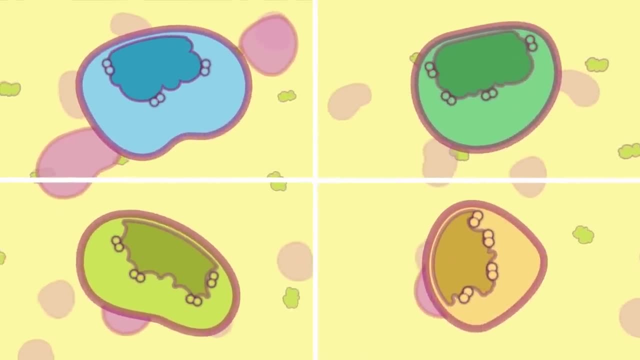 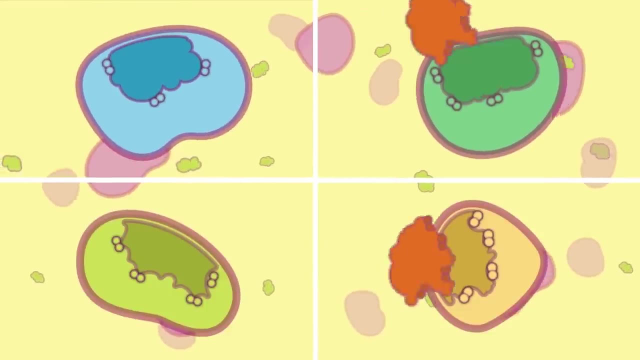 Active site has a specific size, shape and chemical behavior rendered to it by specific arrangement of amino acids. Thanks to these amino acids, an enzyme's active site is unique only to a particular substance. There's no specific spot where the enzyme can cause any reaction, so the enzyme's active site is in the active site. 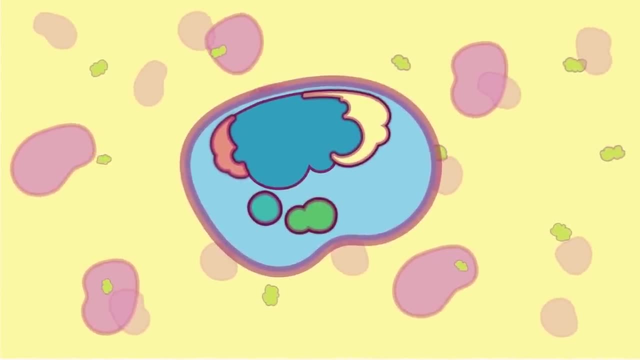 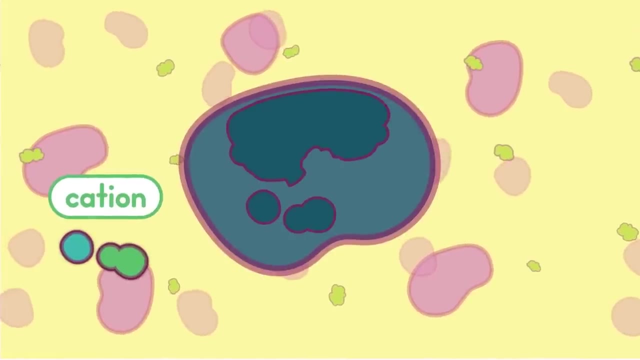 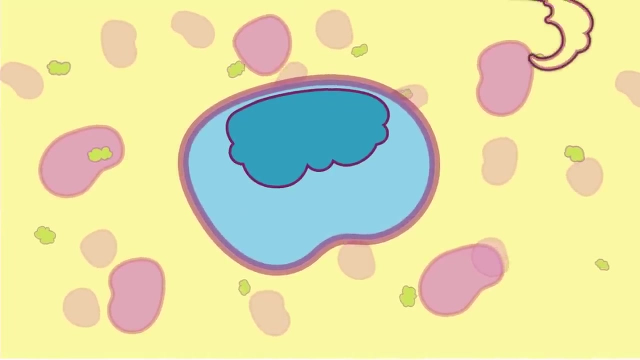 In addition to the active site, many enzymes consist of a non-protein part called cofactor. Cofactors may be cat ions, positively charged metal ions bound temporarily to the active site to activate the enzyme, organic molecules, vitamins or vitamin products that join enzyme-substrate complex, temporarily prosthetic groups, permanently end-greasing proteins and all other factors. 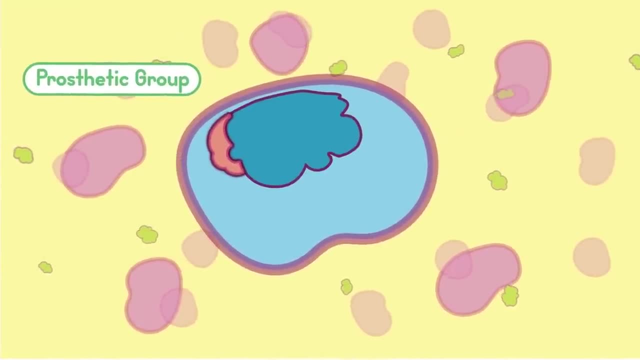 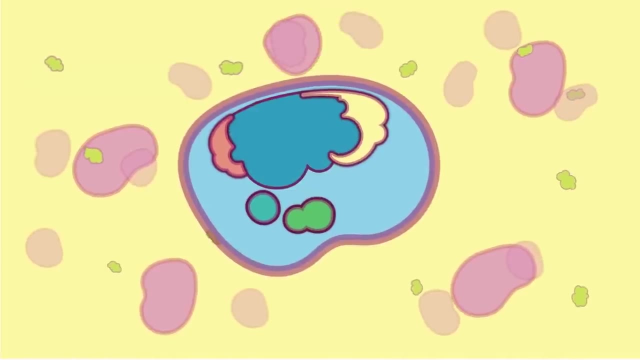 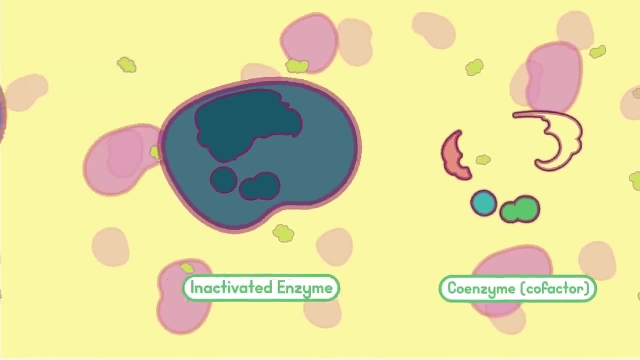 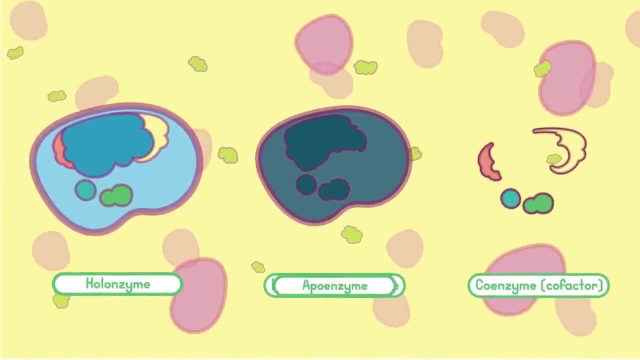 maya. Many enzymes only perform their catalytic role when associated a coenzyme. An inactivated enzyme. protein, along with its coenzyme, non-protein, makes up a system called holoenzyme. To add to the complexity, scientists termed this inactivated enzyme as apoenzyme. 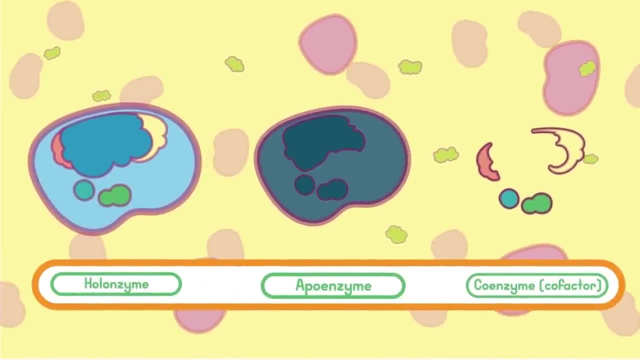 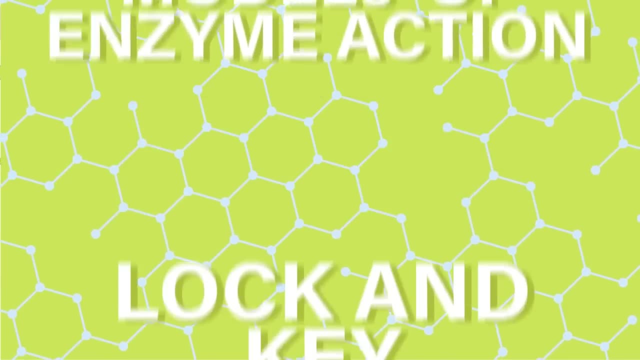 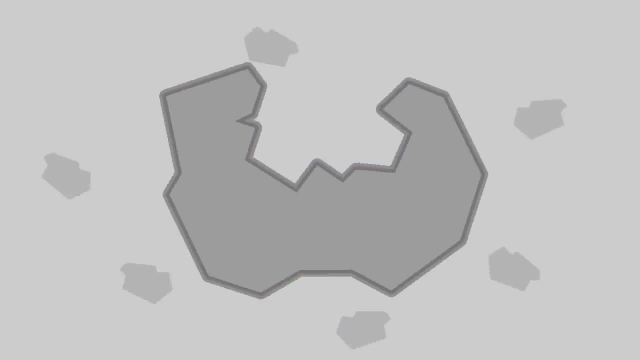 And therefore the equation becomes: holoenzyme equals apoenzyme plus coenzyme. Models of enzyme action: Lock and key hypothesis. This is the simplest model to represent how an enzyme works. The substrate simply fits into the active site to form a reaction intermediate. 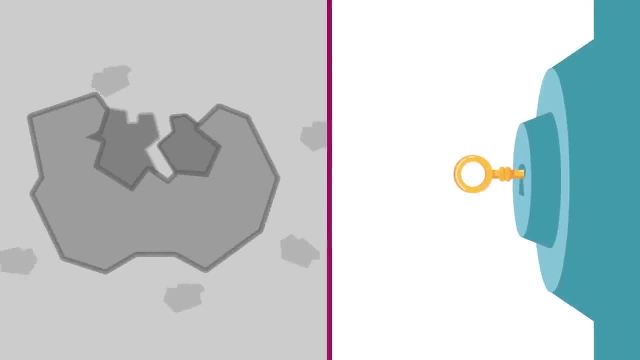 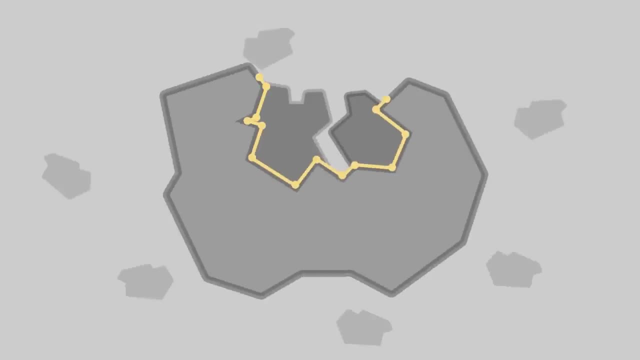 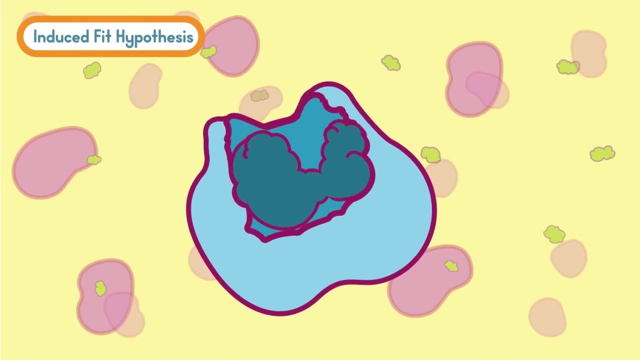 Just like the key fits in its specific lock. the shape isn't changed here. Rather, the structure of the substrate absolutely complements the structure of the enzyme, Like puzzle pieces Induced fit hypothesis. In this model, the enzyme, upon binding of substrate, changes shape. 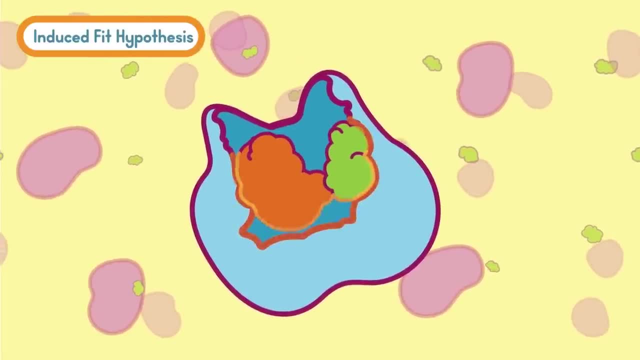 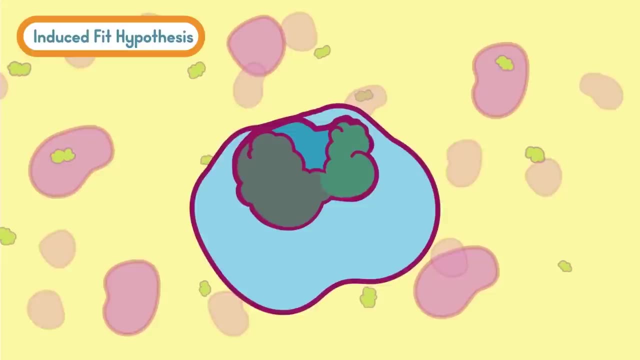 The matching between an enzyme's active site and the substrate isn't just like two puzzle pieces fitting together. Rather, the enzyme changes shape and binds to its substrate even more tightly. This fine-tuning of the enzyme to fit the substrate is called induced fit. 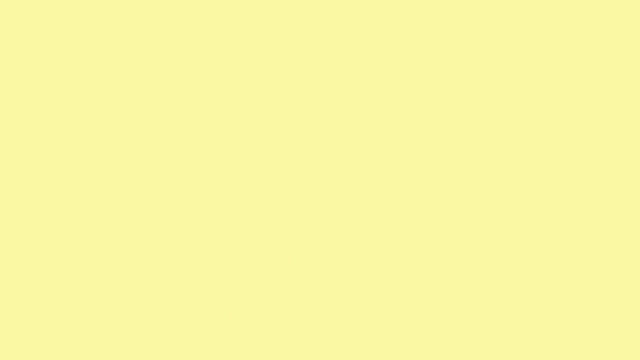 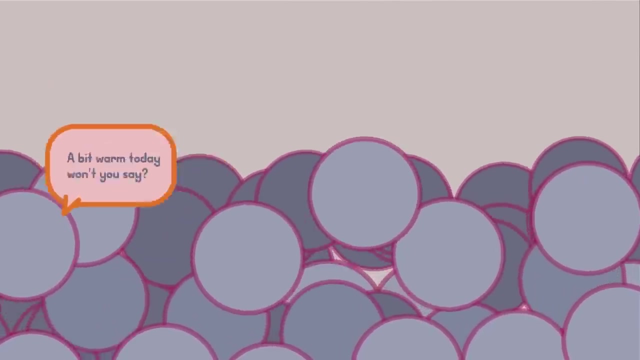 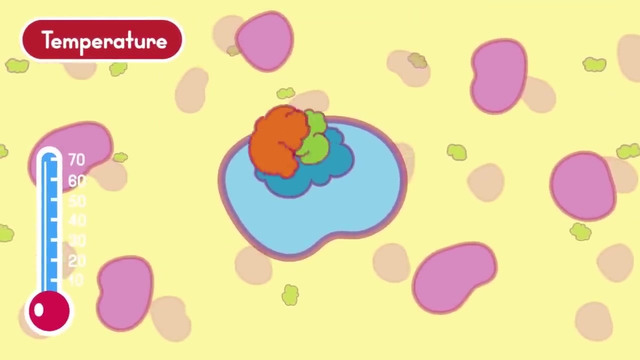 Environmental effects on enzyme function. Active sites are very sensitive. They sense even the slightest change in the environment and respond accordingly. Some of the factors that affect the active site and, consequently, enzyme function include Temperature. The suitable temperature for enzymes to function properly is 37 degrees Celsius.